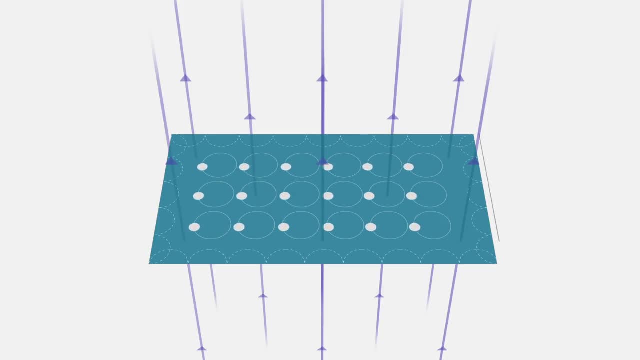 the orbits become open, connected, and they all point in the same direction. So electrons can jump from one orbit to the next and travel all the way around the edge. This means that the material conducts electricity around the edge, but not in the middle. 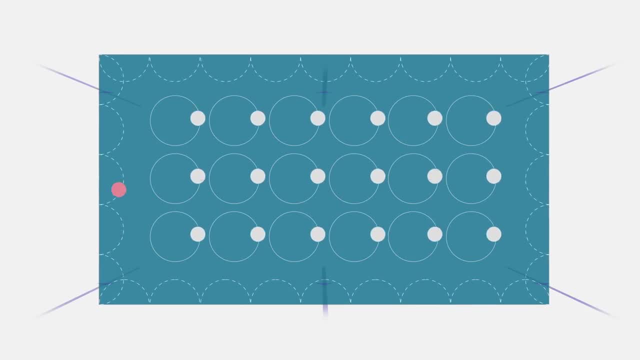 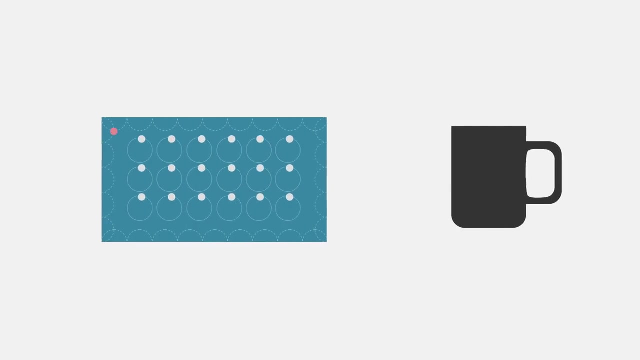 Here's where topology comes in. This conductivity isn't affected by small changes in the material like impurities or imperfections. That's just like how the hole in the coffee cup isn't changed by stretching it out. The edge of such a topological insulator has perfect electron transport. 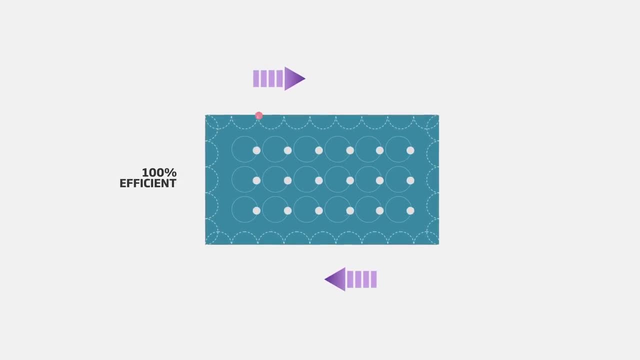 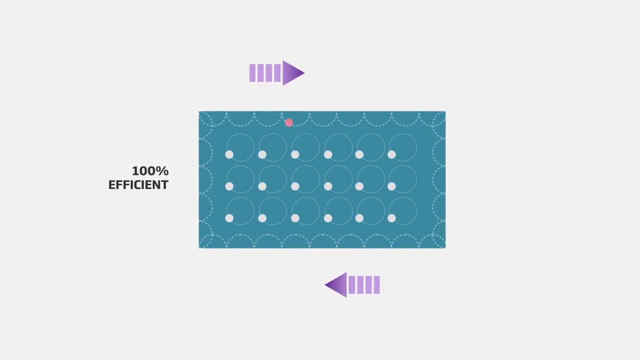 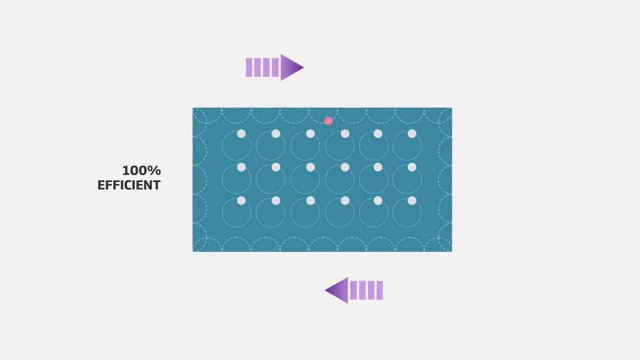 No electrons travel backward, no energy is lost as heat, and the number of conducting pathways can even be controlled. The electronics of the future could be built to use this perfectly efficient electron highway. The topological properties of subatomic particles could also transform quantum computing. 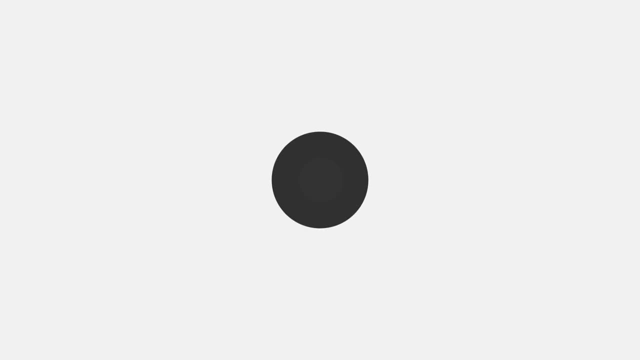 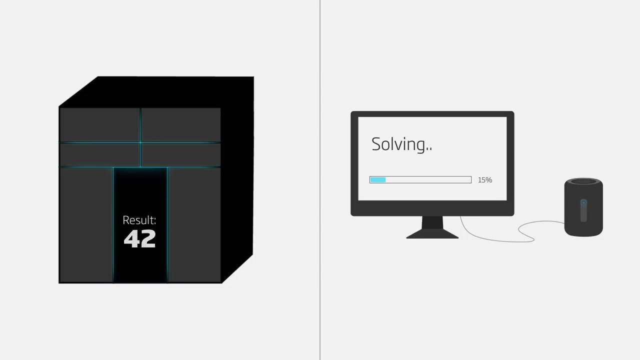 Quantum computers take advantage of the fact that subatomic particles can be in different states at the same time to store information in something called qubits. These qubits can solve problems exponentially faster than classical digital computers. The problem is that this data is so delicate. 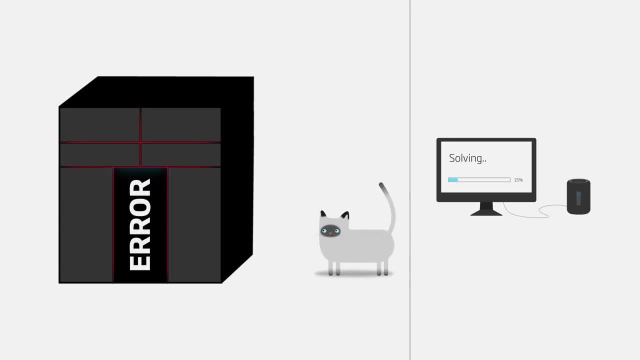 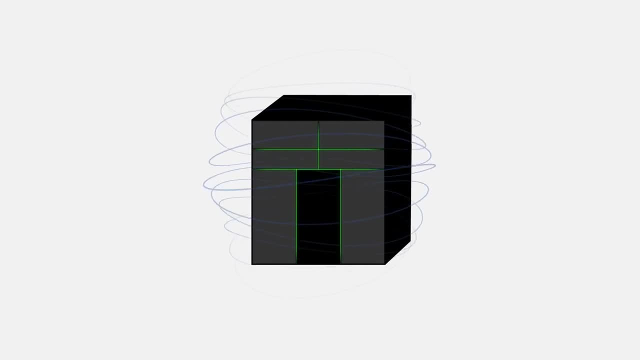 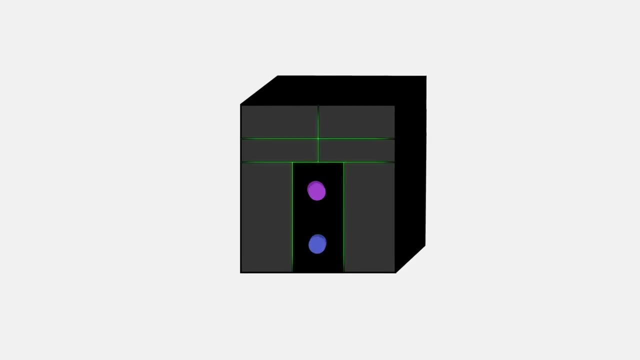 that interaction with the environment can destroy it. But in some exotic topological phases the subatomic particles can become protected. In other words, the qubits formed by them can't be changed by small or local disturbances. These topological qubits would be more stable. 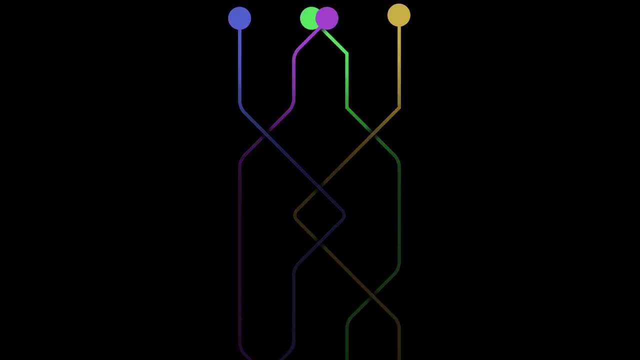 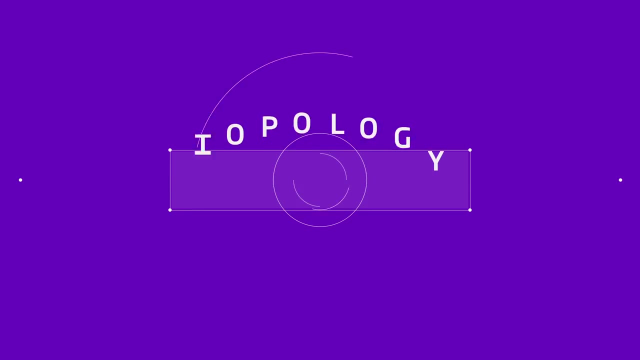 leading to more accurate computation and a better quantum computer. Topology was a real challenge for quantum computers, but it was originally studied as a branch of purely abstract mathematics, Thanks to the pioneering work of Thouless, Haldane and Kosterlitz. 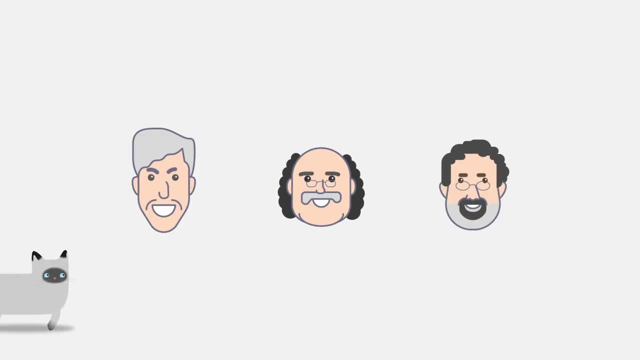 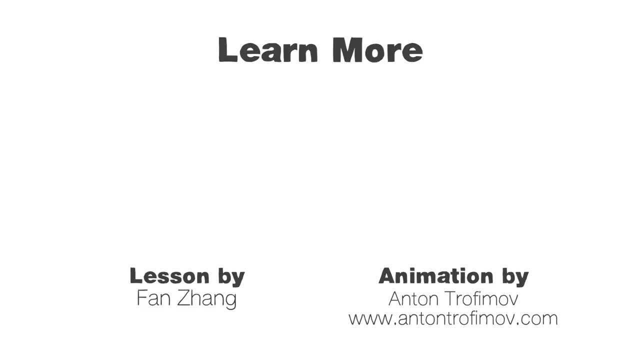 we now know it can be used to understand the riddles of nature and to revolutionize the future of technologies. Subtitles by the Amaraorg community.